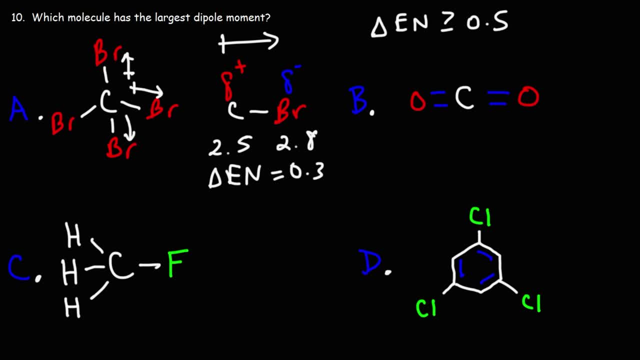 is relatively small, but notice that all four outer atoms of this molecule are the same. for this tetrahedral shape all of the dipole moments will cancel because the arrows they're all pointing in opposite directions. so the dipole moment for carbon tetra bromide is going to be zero. it is completely nonpolar now. 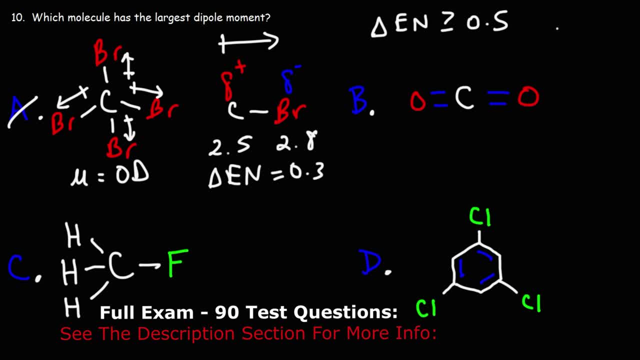 looking at answer choice B, carbon dioxide. the carbon-oxygen bond is highly polar. oxygen has an electronegativity value of 3.5, so the EN difference is 1. so that's a polar bond. but the dipole moments. they cancel because there's two carbon-oxygen bonds that point in opposite direction. there's 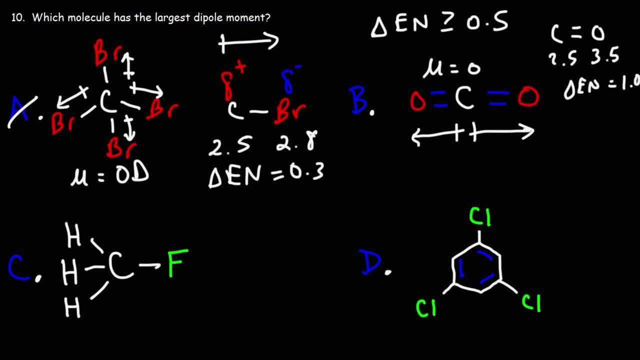 going to be no net dipole moment. so even though this dipole moment is nonpolar, the dipole moment is nonpolar. so the dipole moment this molecule has polar bonds, the molecule overall is nonpolar because the dipole moments cancel. now look at an answer. choice D: the carbon-chlorine bond. 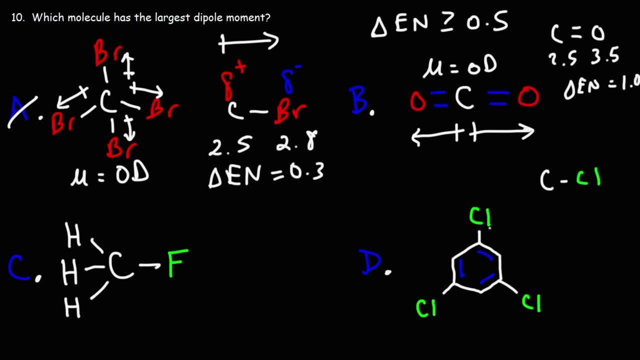 that bond is a polar bond. chlorine has an electronegativity value of 3.0, so we have an EN difference of 0.5. so it's just on the threshold. now, if we were to draw the dipole moments for carbon-oxygen bonds, we're going to have to. 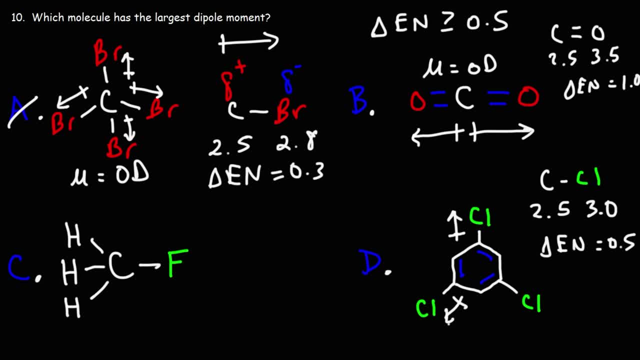 draw the dipole moments for the carbon-chlorine bond. notice that the arrows they all point in opposite directions. so if you were to draw them like vectors, the error at the top it's going in the positive Y direction. then we have an arrow in this direction and one in that direction. now the two arrows. 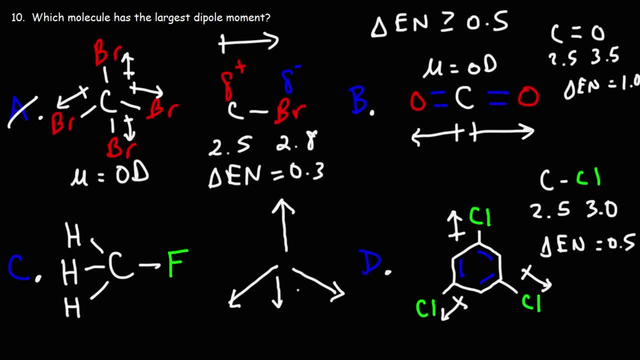 at the bottom. they both have a Y component that goes in a negative Y direction. the one on the right has an X component and the one on the left has an X component going to the left. the X components they cancel because they're opposite to each other. the two Y components they're. 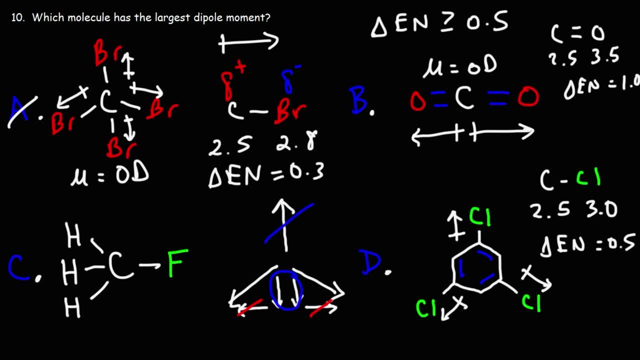 additive but they cancel with the vector on top. so all of the X and Y components cancel. therefore the dipole moment of 1, 3, 5 triclosan benzene is zero. overall that's a non polar molecule. now looking at carbon fluorine, that bond is very polar. fluorine has an electronegativity value. 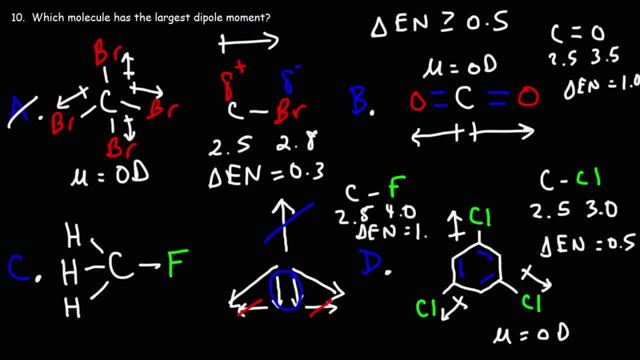 of 4.0. so the EN difference is 1.5. so we're dealing with a highly polar bond. the dipole moment is going to go towards the electronegative fluorine atom. now, if you look at the carbon hydrogen bond, it's nonpolar, but the EN 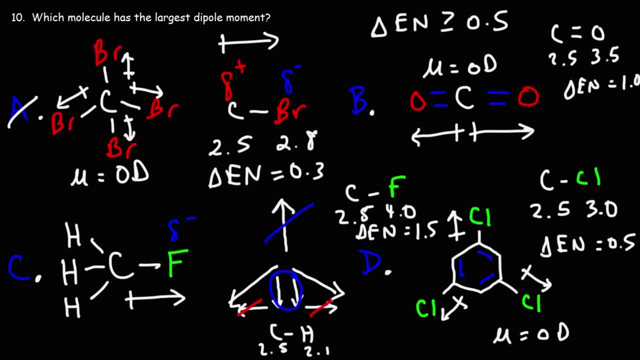 difference is 0.4. so you do have a small dipole moment there. the arrow is going to point towards the more electronegative carbon atom. so we have a dipole moment here going towards the carbon atom, a small dipole moment here as well. and 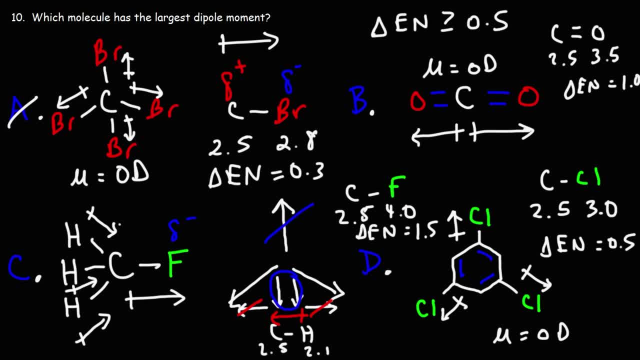 another one. now notice that the Y components of these two will cancel. this one has an upward Y component and this one has an upward Y component. this one has a downward Y component. but the X components of each of these three vectors? generally they're towards the right. each of them has an X and pointed.